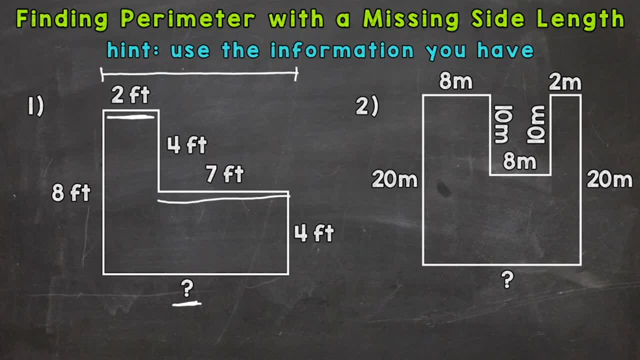 and it's going to be this: seven feet here. If we have that seven feet plus that two feet, that's going to match that bottom side. So two feet plus seven feet gives us nine feet. Now we have all the information we need in order to calculate. 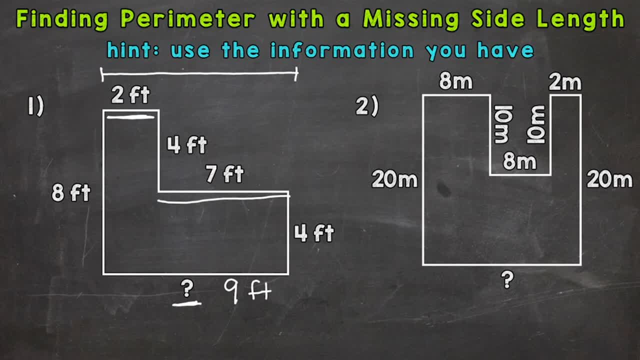 Perimeter. so let's add up all of the sides and I'm going to start with the two feet up top. So two feet and I crossed it off. that way I don't count anything twice or forget to add any of the sides. Then we have four feet. 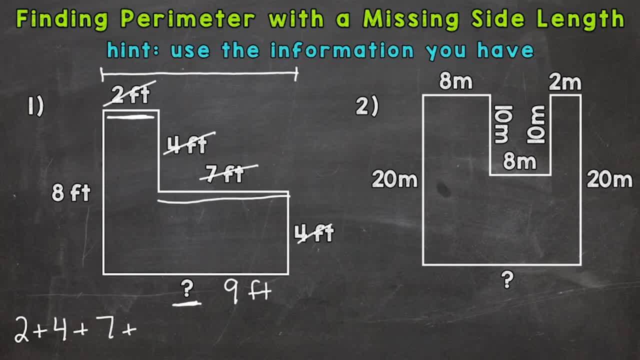 plus seven feet, plus four feet, plus nine feet and lastly, plus eight feet. We can always double check to make sure we got everything. So one, two, three, four, five, six sides and we have one, two, three, four, five, six measurements that we're going to add up. 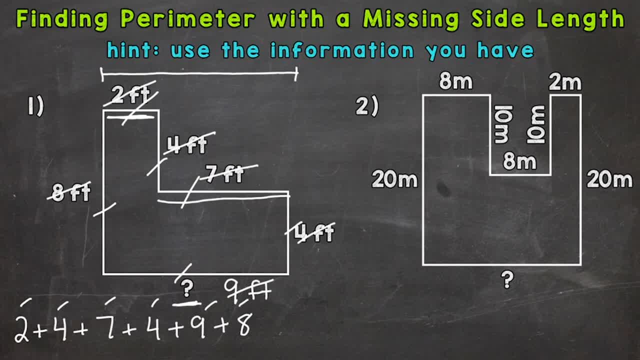 So we're good to go. Two plus four is six plus seven is thirteen plus four is seventeen plus nine is twenty. six plus eight equals thirty four, and our unit of measure is feet, So our perimeter equals 34 feet. So let's go to number two. where again our missing side length. 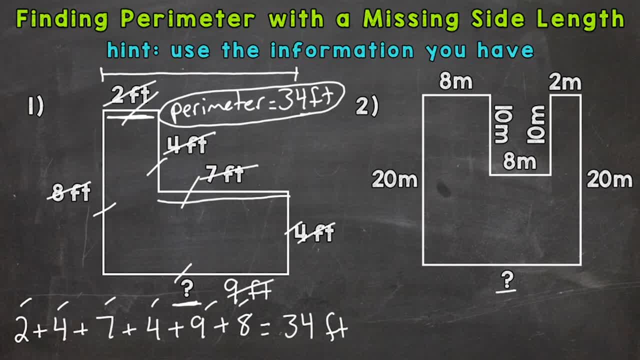 is at the bottom. So let's take a look up top and we have eight meters here. We're going to use this and remember we need to go all the way across. So if we take a look at that eight meters and this two, that doesn't quite go all the way across because we have this gap here. 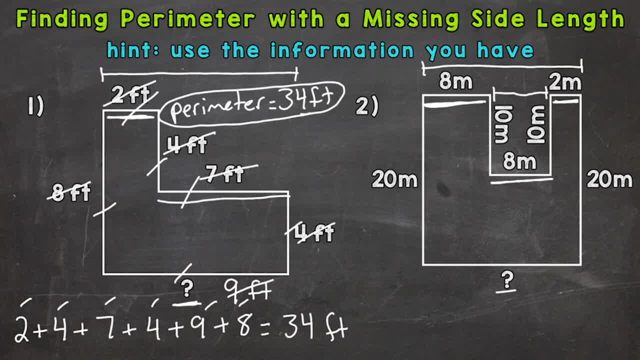 So let's look down here and we have another eight meters. So this eight plus this eight plus that two will give us all the way across, which matches our missing side length. So eight plus eight is sixteen plus two is eighteen, So our missing side length is eighteen meters. Now we're good to go as.